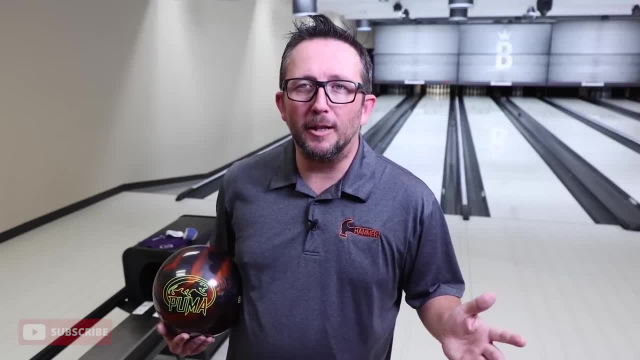 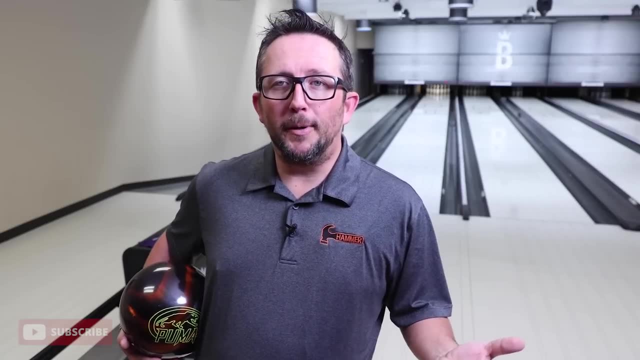 way across the board, pretty much every single ball that goes 12, 13 pounds, with a few exceptions on the entry level. But this is the only ball we had in the factory- actually in our warehouse right now, So I grab this. I know it's a little bit older but the concept remains the same. So original Puma had. 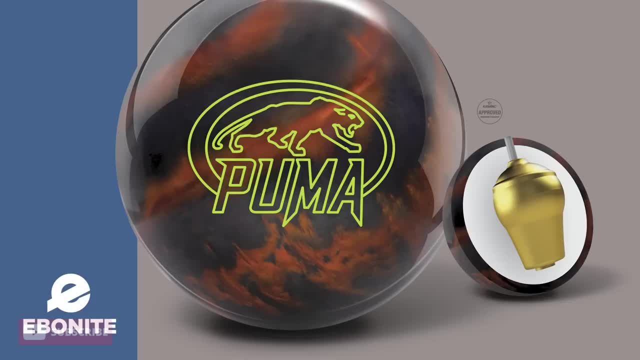 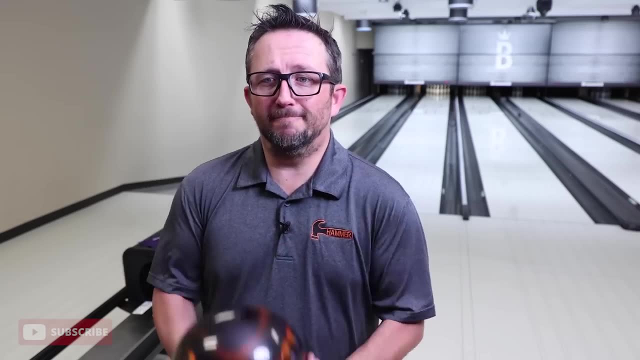 a differential of around 036 with a much lower RG. This one has a higher RG but a little bit more diff with the 040.. So I'm going to throw 12 pounds in this video. You know this is very light. We're gonna see if I can strike consistently. So I don't know what I'm bowling. 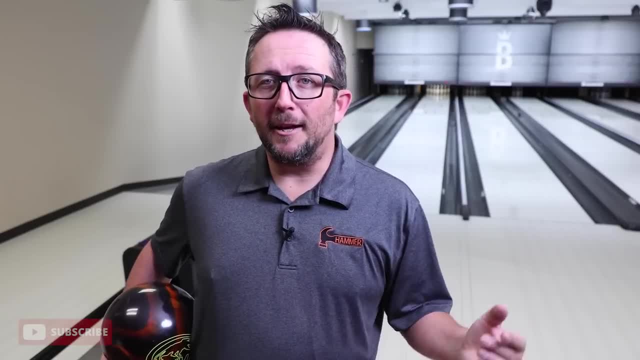 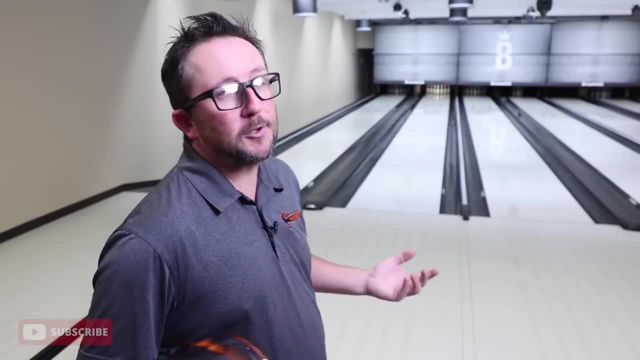 on The board says crown jewel, but that was as of yesterday. They've been bowled on. so this is the perfect test. Can I strike with twelve pounds? We're going to find out. I haven't thrown a single shot. I haven't thrown any warmups. I figure throwing a 12 pound ball is kind. 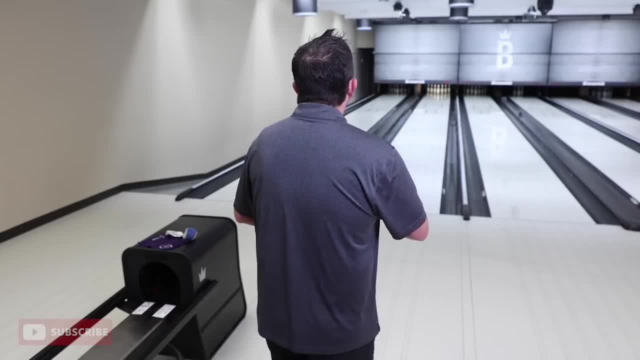 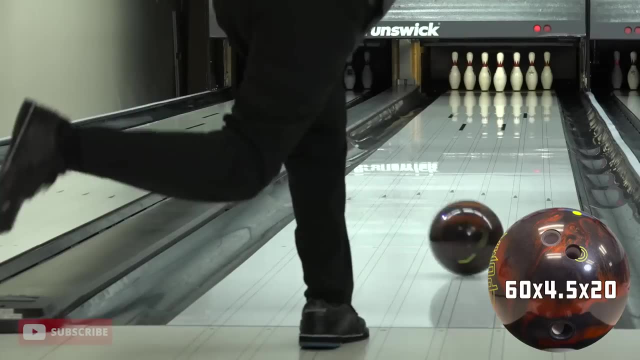 of like a warm up anyway. So we're gonna try it all different angles, like we always like to do, and see what 12 pounds can do for me. Oh my goodness, I can't even feel it in my seat. Oh, I couldn't believe. it actually fell on the ground and the ball lands on me. That's antibiotics, and 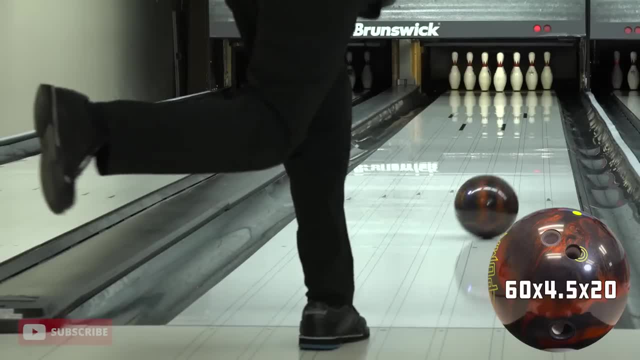 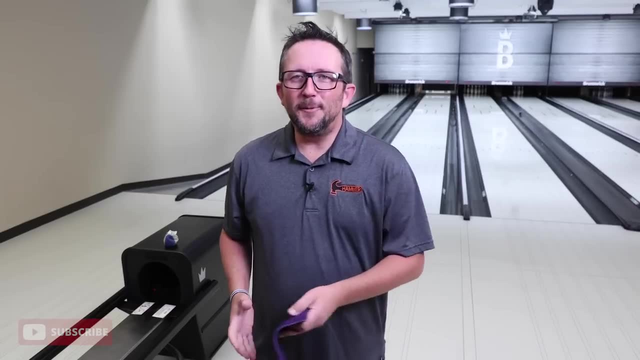 I'm so sorry about that. Can I strike with 12 pounds? I don't know. Can I strike with 12 that in my arm swing? That's gonna take some getting used to, But that's why we're here. So as you get older, it's almost inevitable. 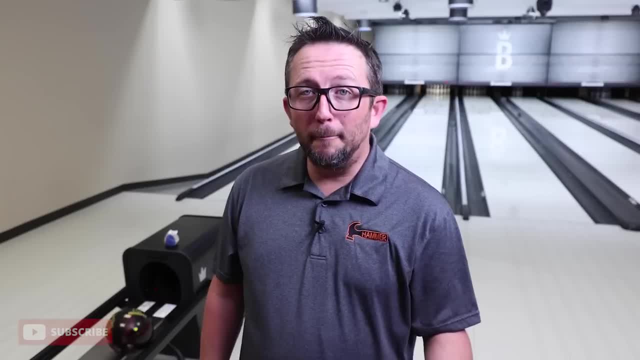 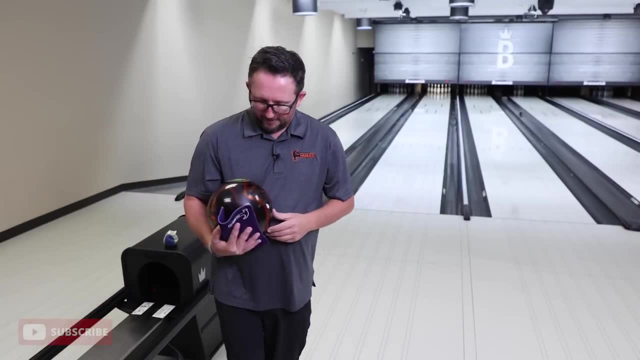 you're probably gonna have to drop weight. I throw 15 pounds, so going to a 12 pounder, I haven't thrown 12 pounds since I was like 11 years old, So the main things we're looking for here with a ball- like an entry level ball- 12 pounds. 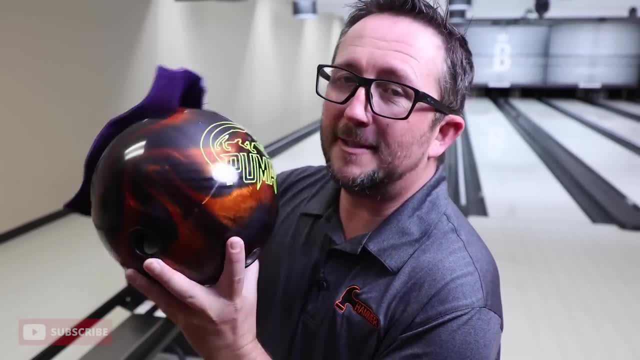 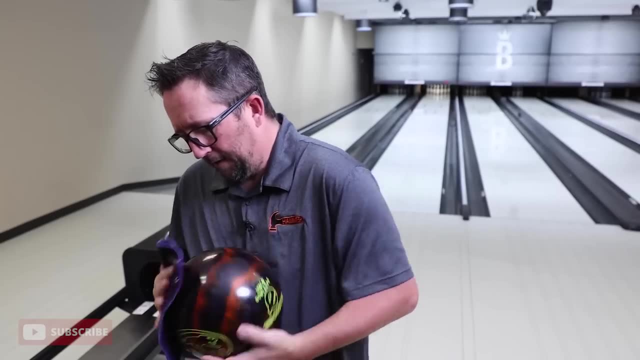 is it gonna flare? And as of that first shot, yes, the separation is about a 3 16ths quarter inch roughly in there, but plenty of flare on this thing. So that's the one thing you gotta look for If you're chopping lighter weight bowling balls. 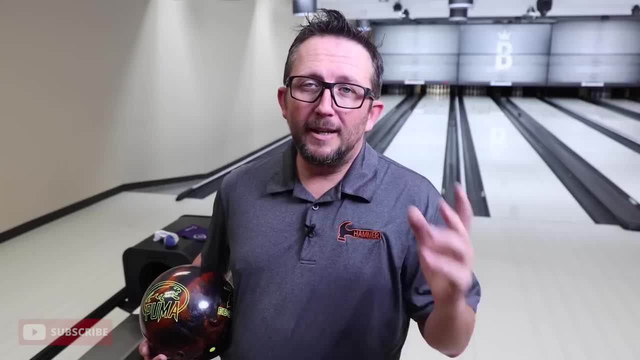 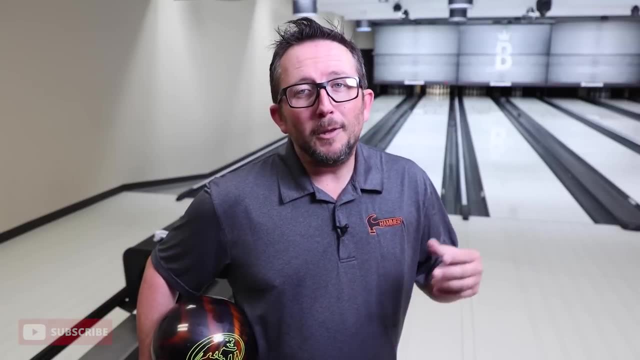 and you like the whatever ball, always pay attention to the numbers. Even if you're looking at a competitor ball, pay attention to the numbers. and if they're using the same shape core, the only way they could do that is with a much lighter density, okay. 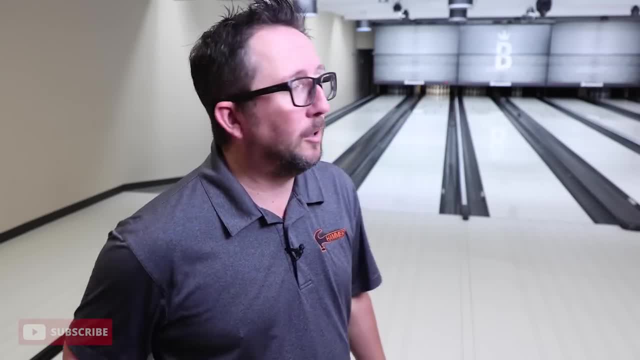 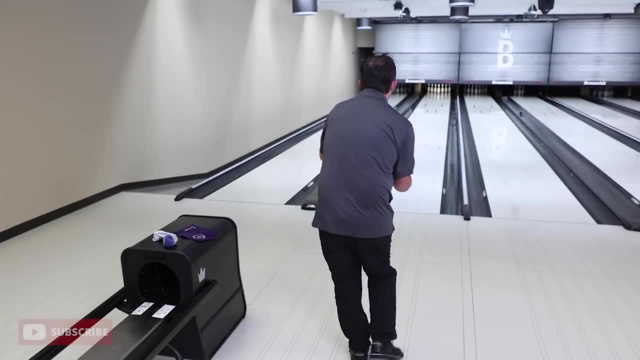 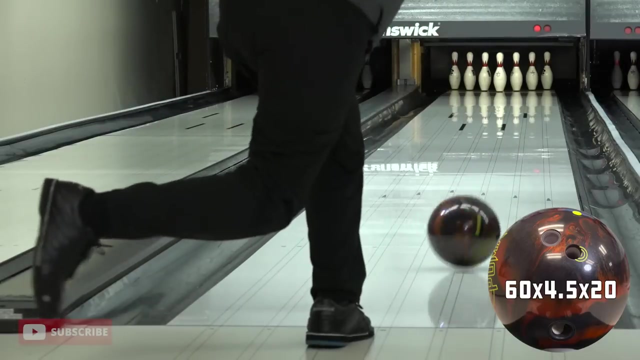 And that's gonna bring the differentials down to a level that's not even close. All right, let's try that again, but first shot I'm gonna keep it in a lot slower than that Pluck, So it's gonna take a little bit of effort. 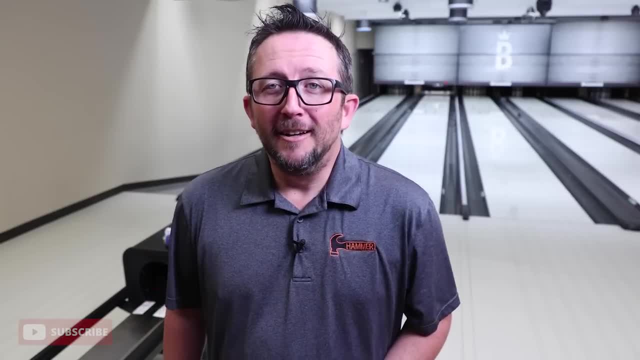 to be able to get a 12 pounder through the pins like I would a 15 pounder, So I'm gonna have to use a little bit more friction. This is gonna be a fun video. This is gonna be a little bit of an effort for me. 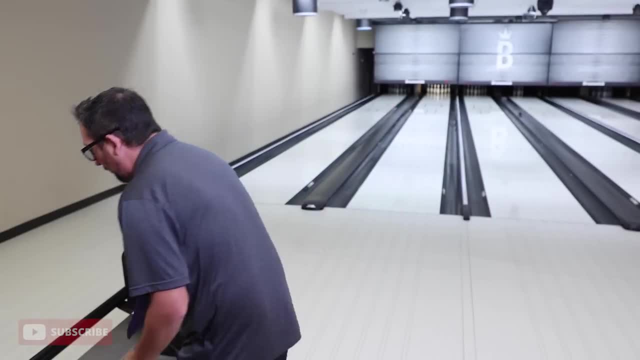 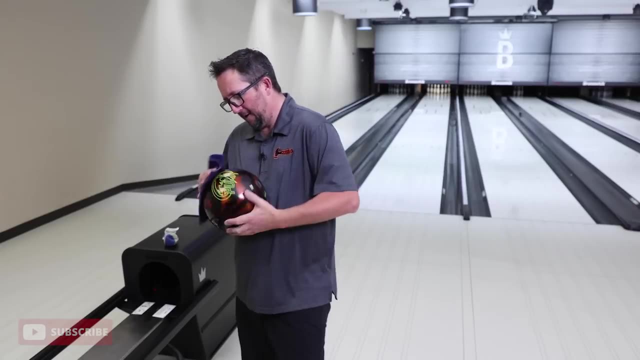 to try to manipulate the ball to be able to do what I need. The ball flares, definitely flares. There's plenty of flare on that. You know this is a very shiny ball. Crown Jewel does have a puddle in the middle. 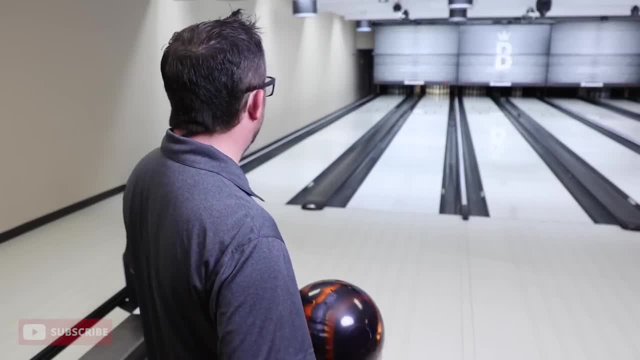 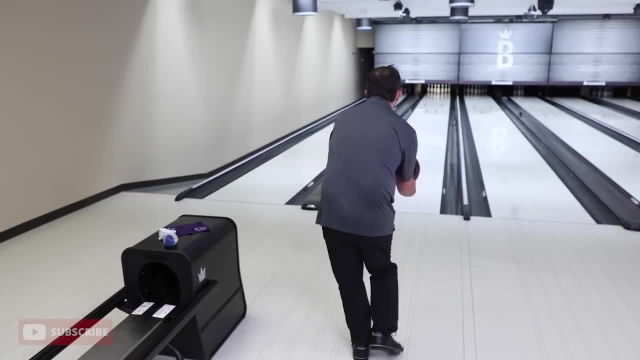 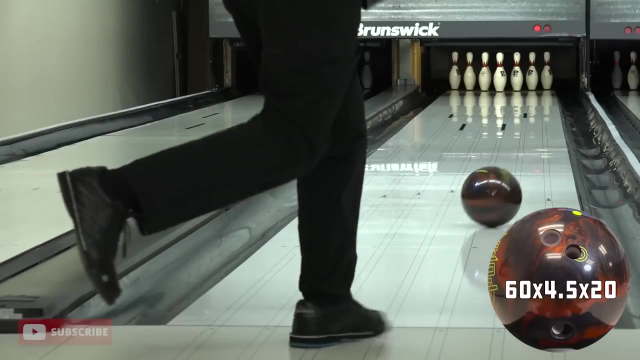 so let's try to throw it outside a little bit, and then we'll start moving in if we need to here. Oh man, Oh, that's hooking. Yes, Totally possible. I knew it was only a matter of time. 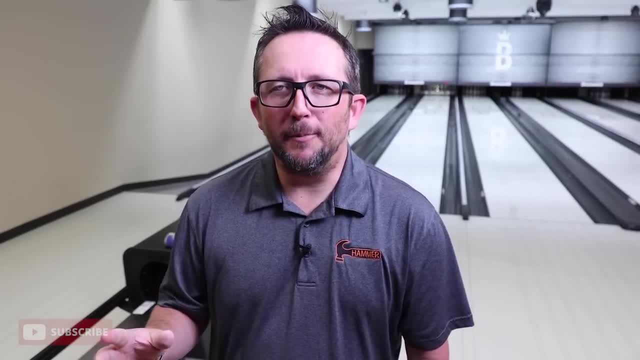 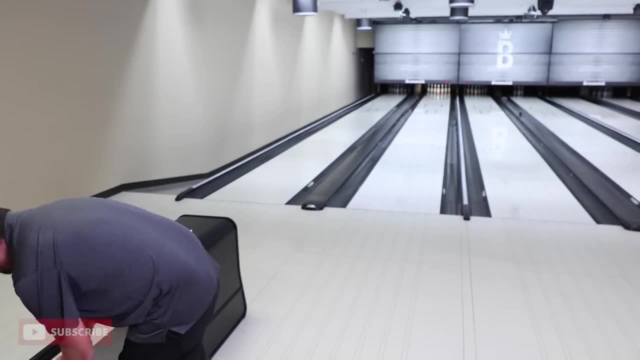 but if you can create entry angle, you can strike with any weight ball On the off-hits lighter weights. that's where you're gonna suffer. But going back to talking about these cores, okay, So why does Brunswick use generic cores? 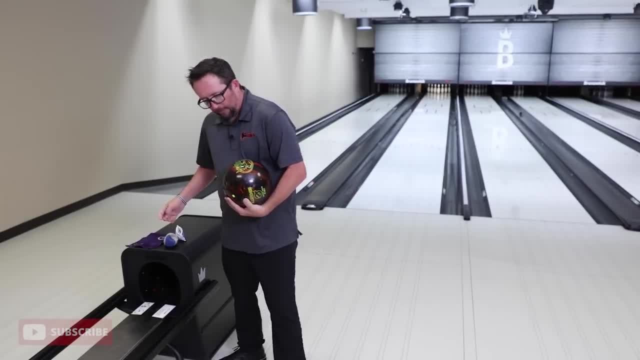 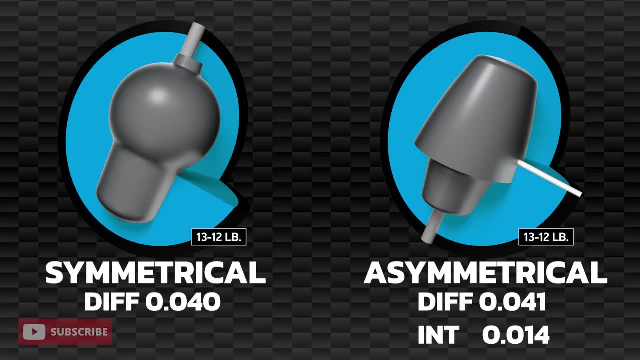 instead of using the same. Because one thing: we've developed lightweight cores that are both symmetrical and asymmetrical. They're both light bulb shape. The lighter weight asymmetrical ball core is gonna be elliptical, It's gonna be stretched, It's gonna be like the old Zone Classic core. 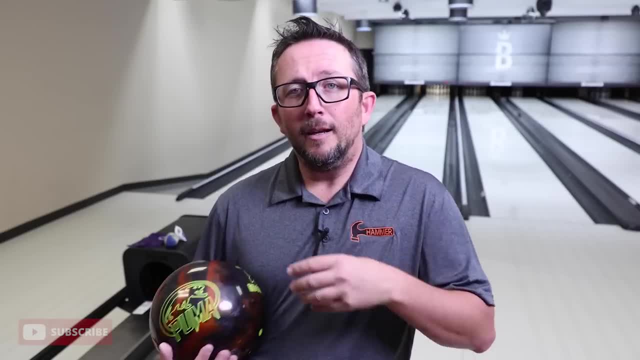 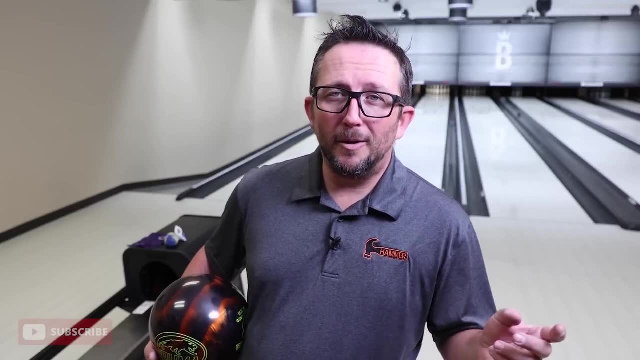 if you guys remember that one- Basically a light bulb that's elongated and give it some asymmetry. So always pay attention to the numbers. You know the most differential you're gonna get out of a 12 or 13 pound ball is gonna be about 040-ish. 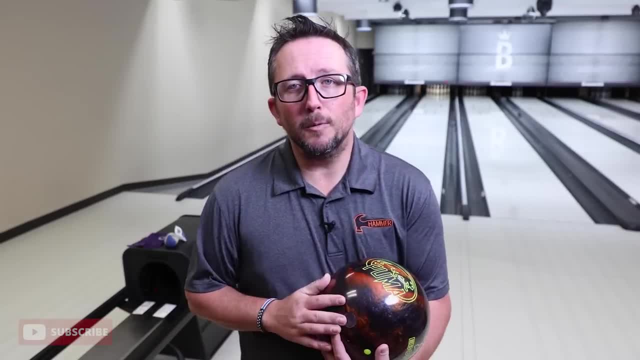 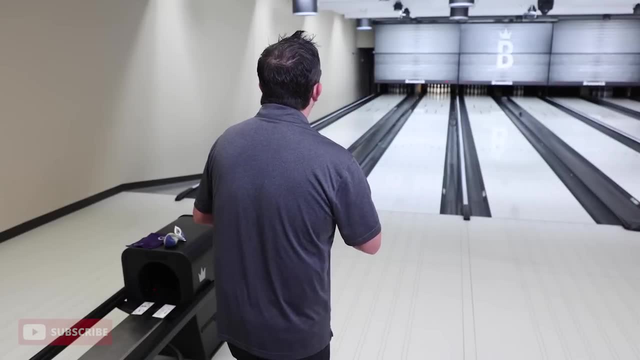 You can't really push the limits too much on that just because there's not a lot of density there to work with. So let's throw a couple more shots. I'm gonna move in a little bit. Remove five left. Let's open the angles up a little bit. 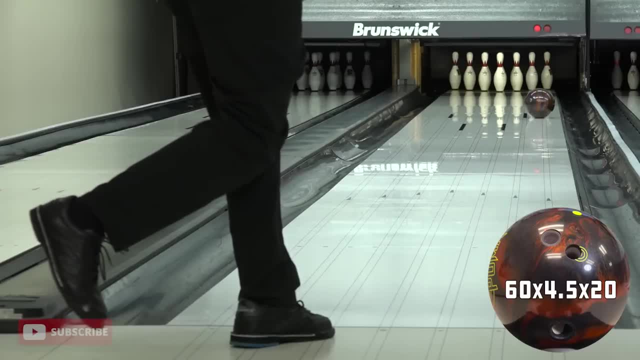 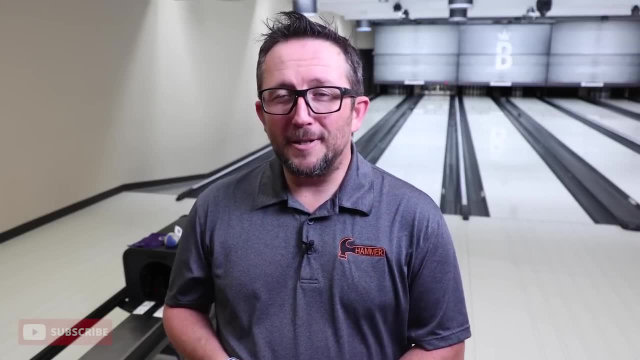 That's a good sign. Wasn't really a flat 10, it kinda wrapped 10 there, So you know there's still good hitting power. You know, if I was suffering from like an injury or say, temporarily, you try to, you know. 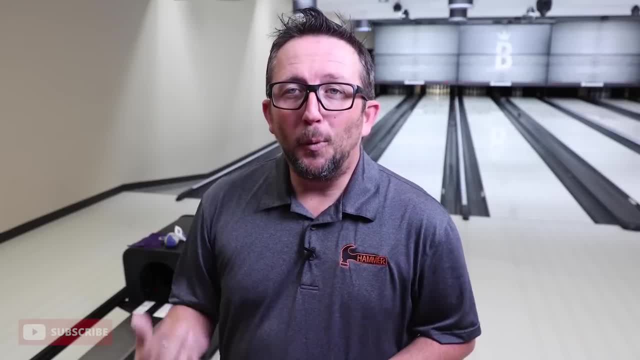 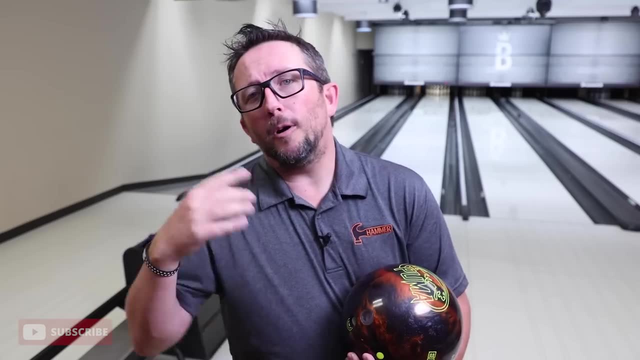 you had an injury in your hand or whatever and you need to work back into the weight. you know you gotta work on. you know flexibility or whatever. It's good to start with a lighter weight ball and bring it back up so you can get back in the game. 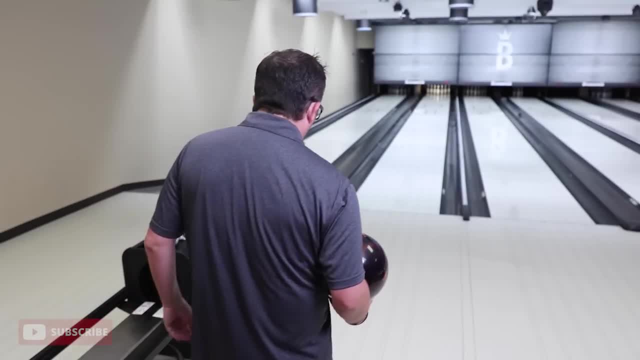 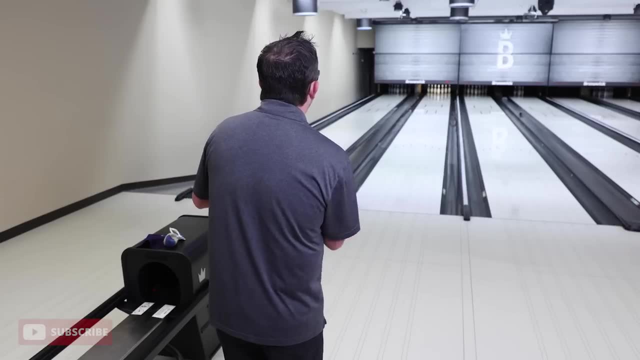 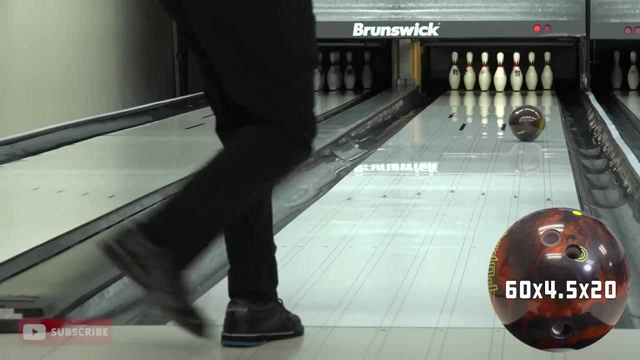 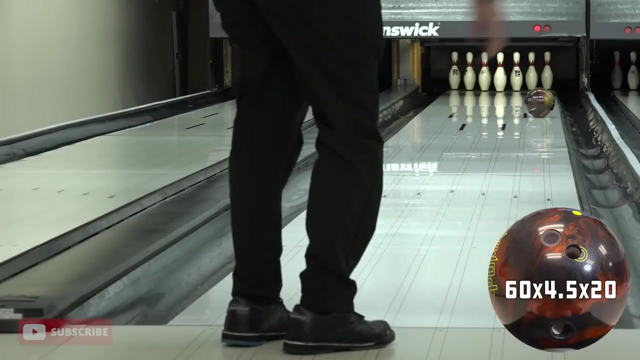 without hurting yourself. So if you use 15, you can make do with a lighter ball, Absolutely can. Obviously, it takes a little bit of thinking to get the timing right, Yikes, Because you know the trigger mechanism is a little bit different. 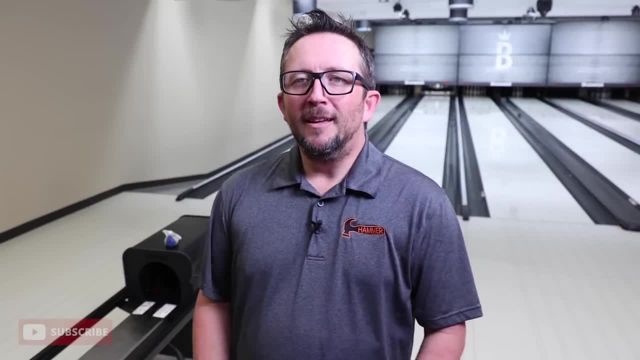 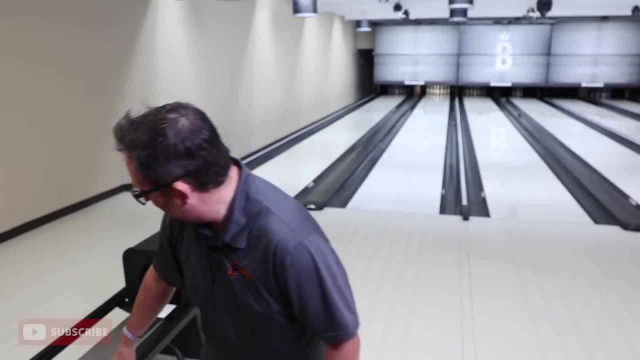 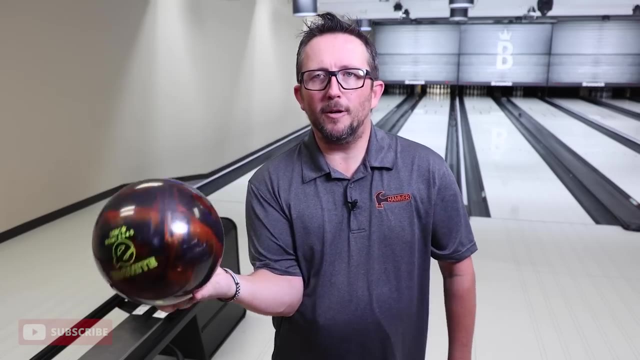 I don't have the extra three pounds at the bottom, but what I do have is the ability to manipulate the ball roll a lot better. I can do this and this with the ball, no problem, Because look like I can't do this with a 15 pound ball. 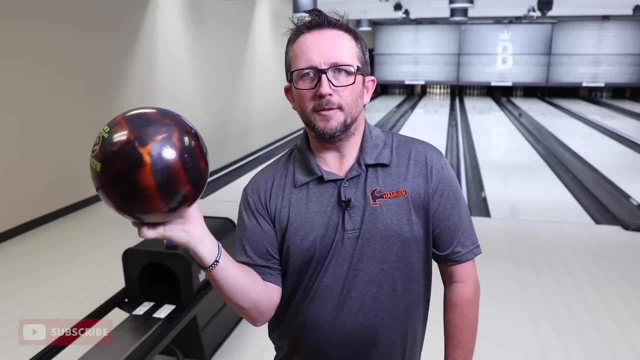 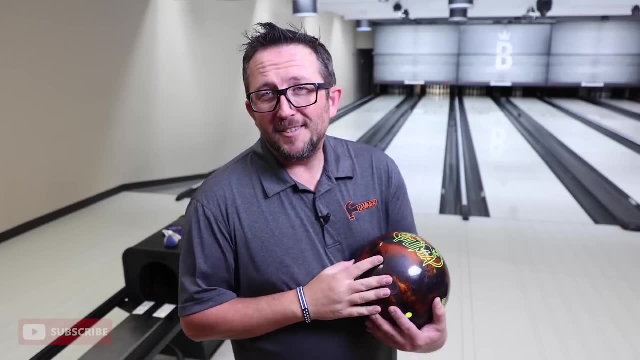 but I can probably easily do this with a 12.. There's no way I'm doing that with 15.. So I'm gonna go with a 12. I can get a lot more on it. I can probably rev the snot out of this ball. 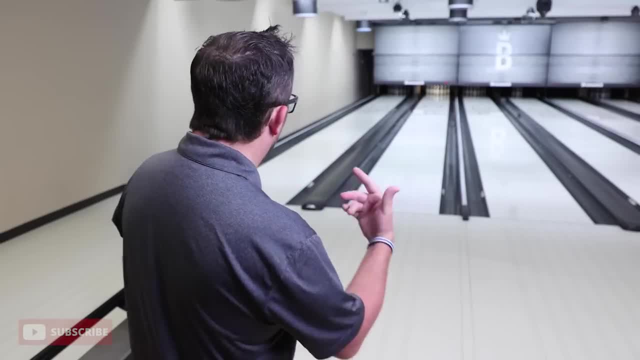 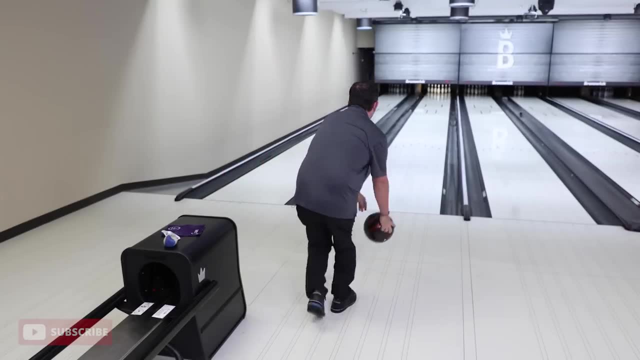 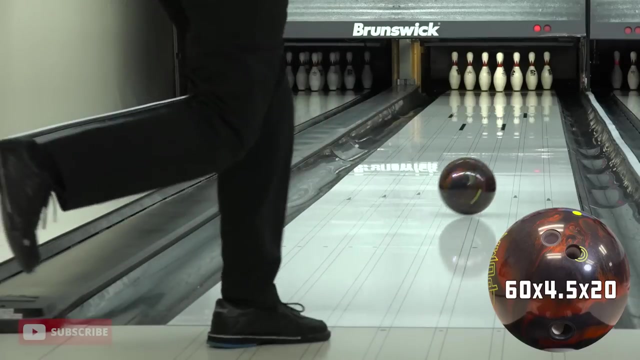 but I'm trying not to. That's the whole thing. Like you can drop down in weight and still have success, and your rev rate probably goes up a little bit. See, Grab it at the bottom. Not a great shot, So obviously I could throw it in the air. 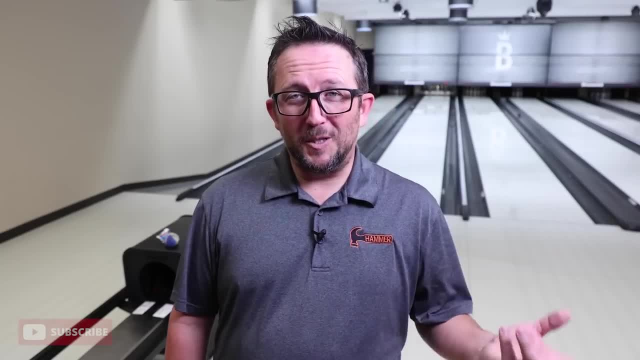 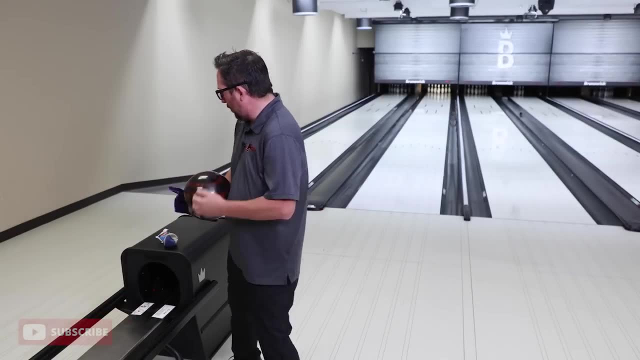 I could throw this a lot harder. It takes more effort for me to throw it slower, but it's just gonna be dialing in timing for me at least to be able to just roll it off my hand like I normally would, but I'm just not feeling the weight. 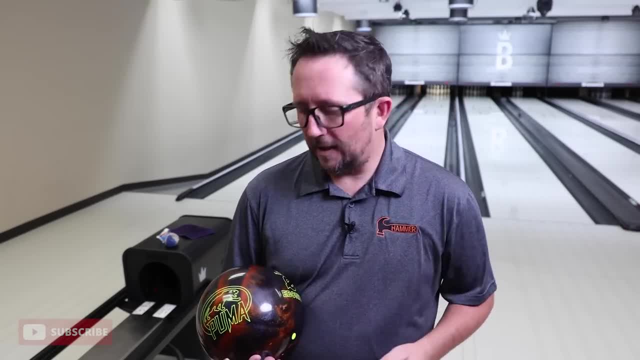 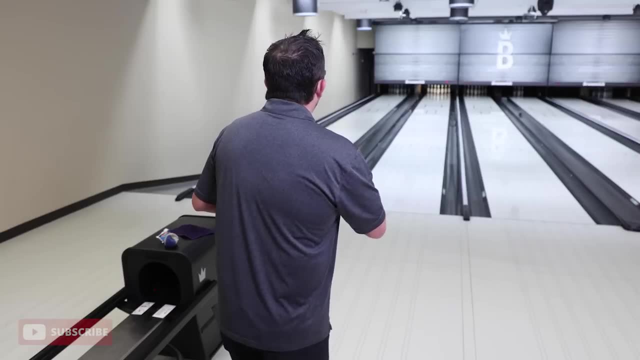 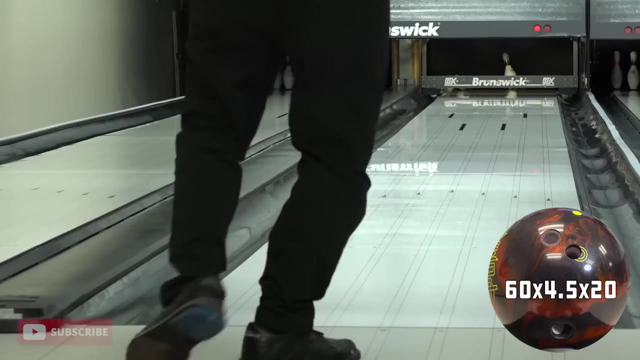 So that's the main thing I see, but not that. the question is: is the performance there? Yes, The shiny ball, it flares quite a bit. It actually is more performance in 12 and 13.. Look at that. Almost left a nine pin with a 12 pound ball. 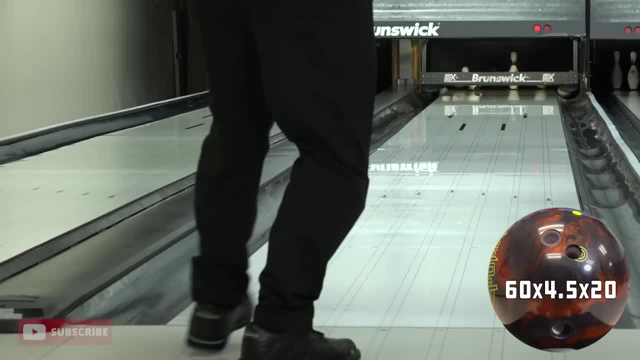 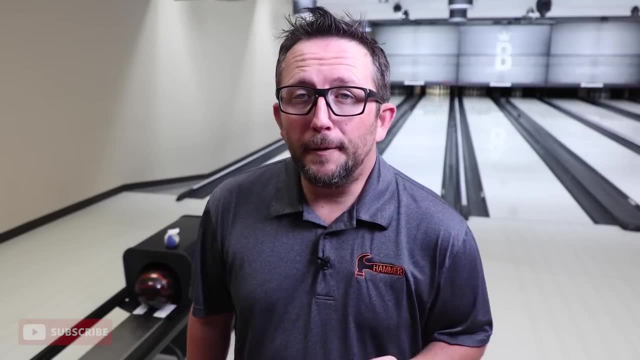 Are you kidding me right now? So when you see these bowling balls that are offered in the 030s, 035, which are a lot of them now, all different brands- if you're throwing 12 or a 13 pound ball, 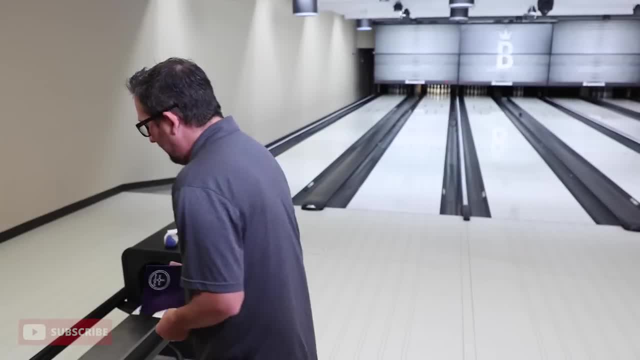 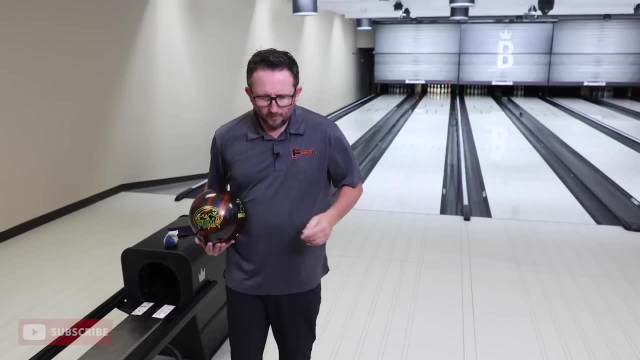 it's actually a little bit stronger core-wise. That's it. So you're gonna get a little extra performance, Not a lot. It's in the same range. You're gonna see 040, no matter what. So, granted, if you're 050, say you know. 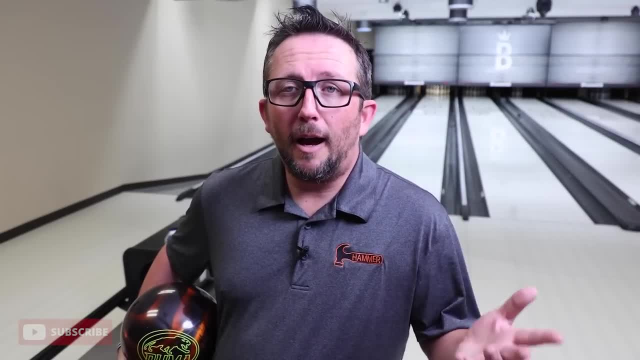 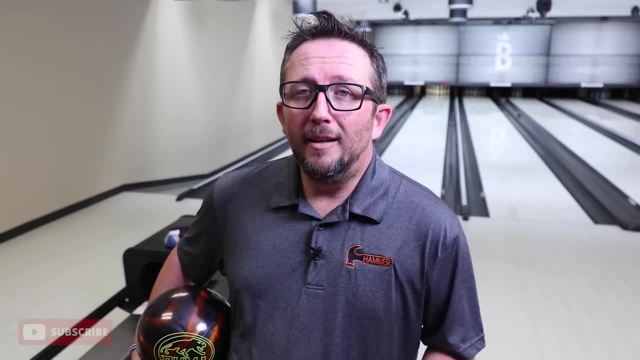 you're looking at Stealth, which is in the 050s. you know you're looking at those higher end Symmetrix. you know you're gonna be giving up a little bit of performance in differential But if you go with the same shape core. 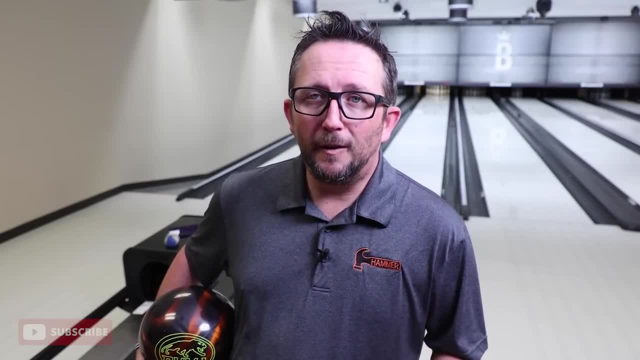 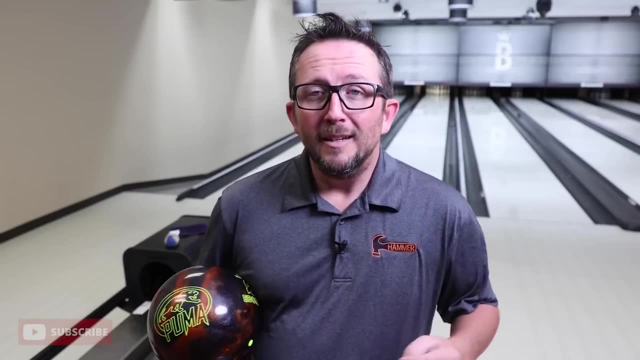 and just change the density, your numbers are gonna drop off significantly. You're gonna be into the nothing. So pay attention to the lightweight numbers. It's the most important part. Obviously, the cover stock is what you're buying. The cover stock stays the same, no matter what weight. 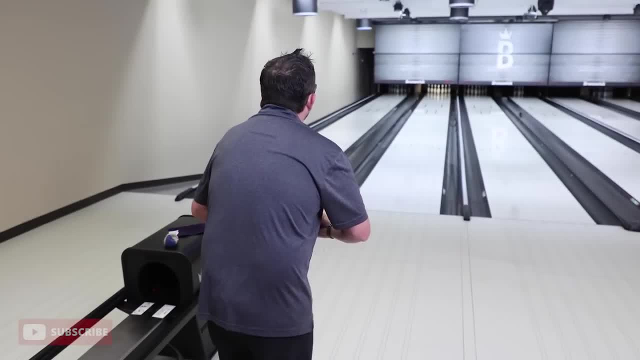 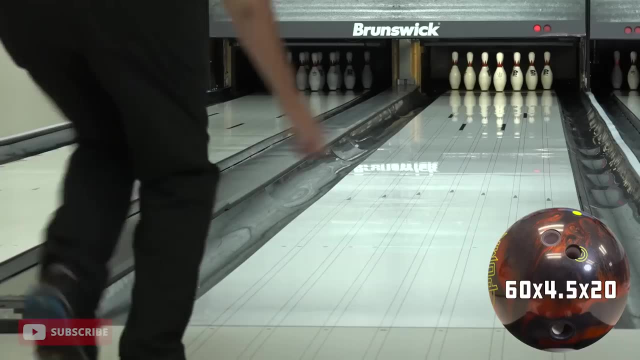 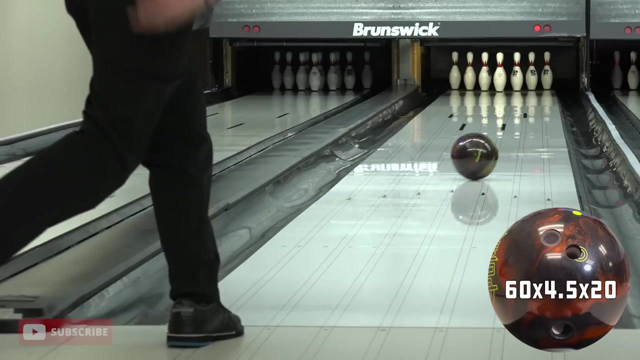 So the core's gonna be the change there. All right, let's try that again. I'm gonna actually move in a little bit more. Five more. Let's try it again. It's really soft. How many times I don't think I've ever seen. 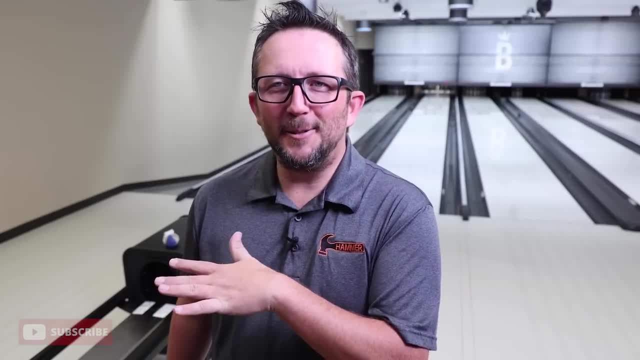 that kind of carry Nine pin falls into the 10 pin. Now, if that was a 15 pound ball, it would've hooked right in Now. if that was a 15 pound ball, it would've hooked right in Now. if that was a 15 pound ball, it would've hooked right in. 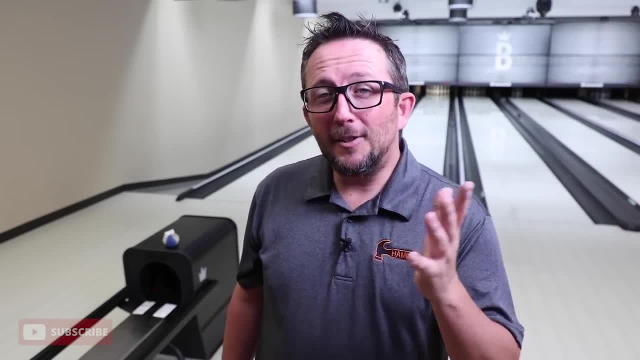 It would've hooked right past the nine pin. It never touched it, But I think the ball actually deflected enough to touch the nine pin as it was going through and splitting the eight nine Fell right into the 10.. So that's hilarious. 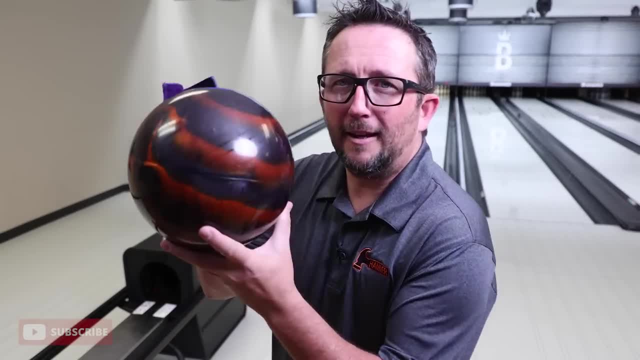 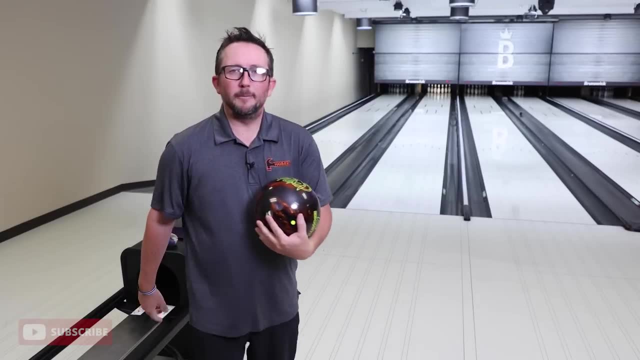 Let's check out the flare on this one, because that was check that out, All the performance you could want. I'm having fun with this. I'm gonna move another five. I'm gonna keep moving until I can't get the ball back. 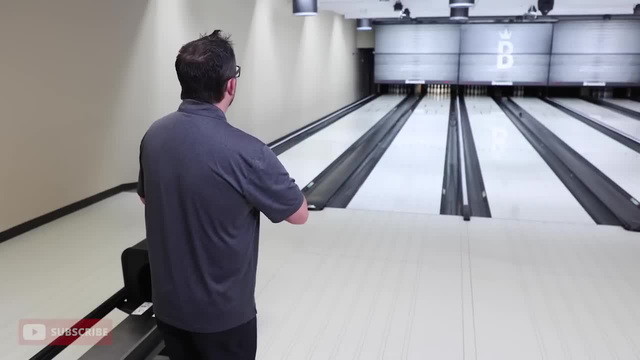 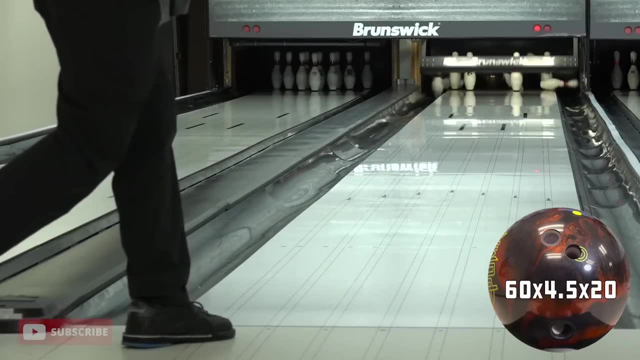 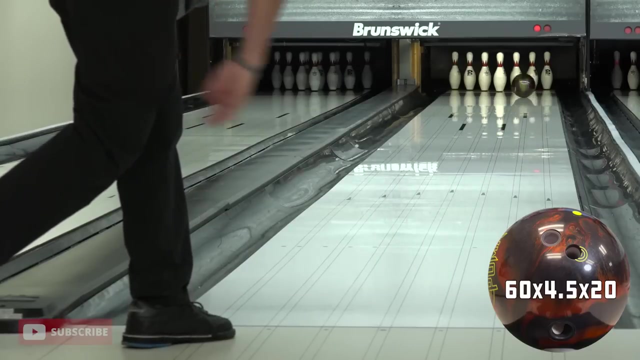 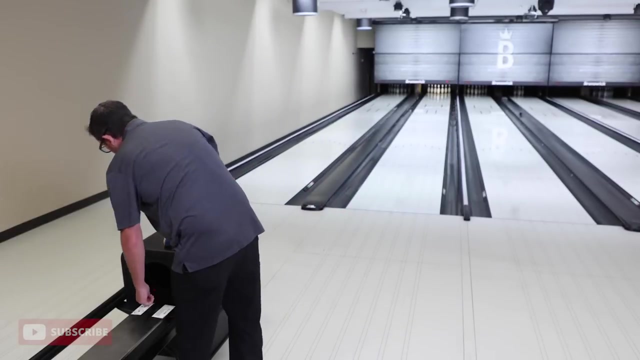 through the pins here. So far, so good. Obviously, speed needs to come down. That could be really good. Maybe I could throw a messenger. How straight would that be? I think I could do it. So, yeah, I mean, that's the whole thing. 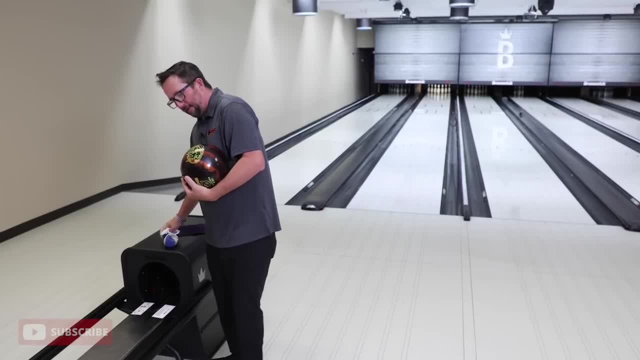 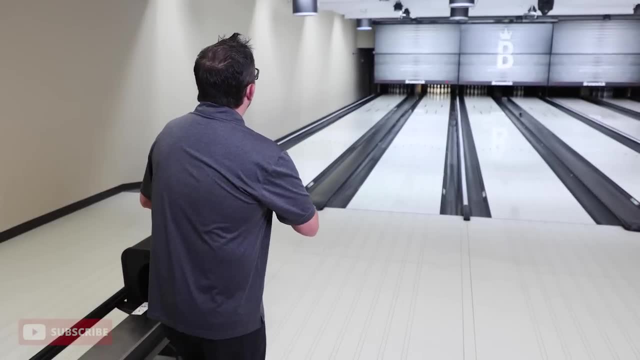